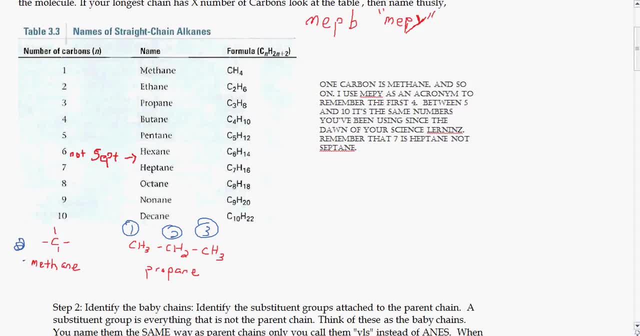 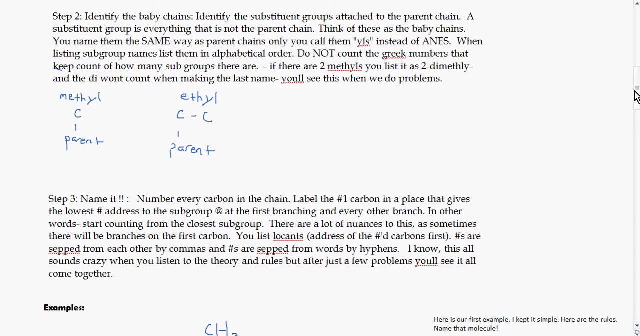 So here I put two examples: Here's methane and here's propane. Here methane only has one carbon hanging out, And here on propane you have three: One, two, three MEP propane. Step two: identify the baby chains. 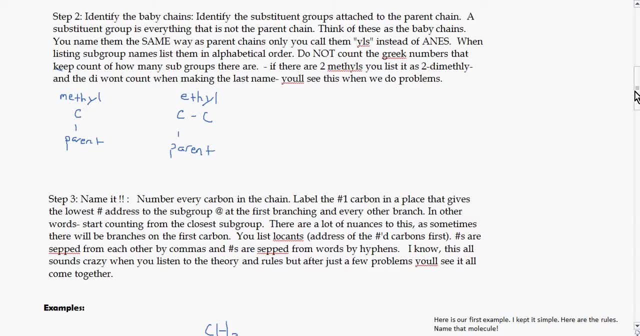 You need to identify the substituent groups that are attached to the parent chain. A substituent group is everything, Everything that is not the parent chain. Think of these as your baby chains. You then name the same way as the parent chains, only you call them ioles instead of aines. 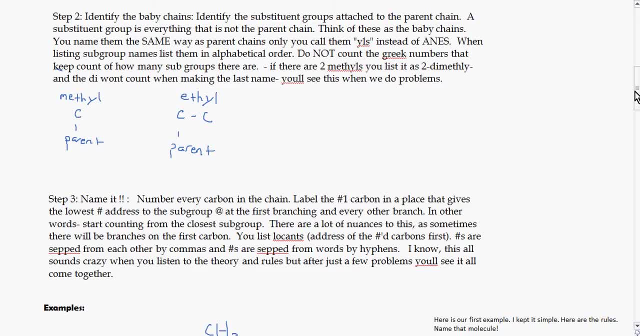 So if you have a single carbon hanging off, that would be a methyl group. Two carbons would be an ethyl group instead of, like, an ethane. So you list these subgroups in alphabetical order and you don't count the Greek numbers that are used to keep how many subgroups there are. 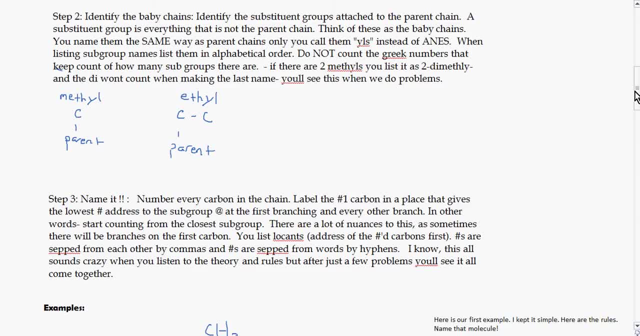 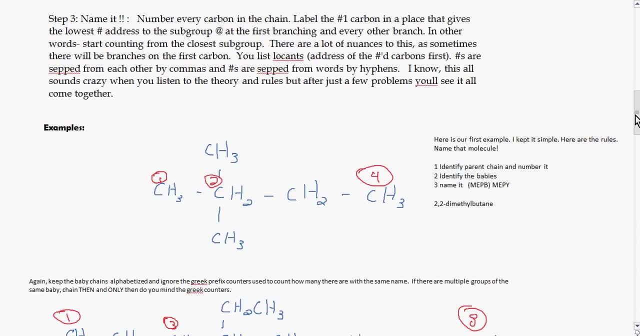 So if there are two methyls, you will list it as two ethyls And you'll see how this applies when we do problems in just a second. And step three: number every carbon in the chain. You want to label the number one carbon in a place that gives the lowest number address to the subgroup. 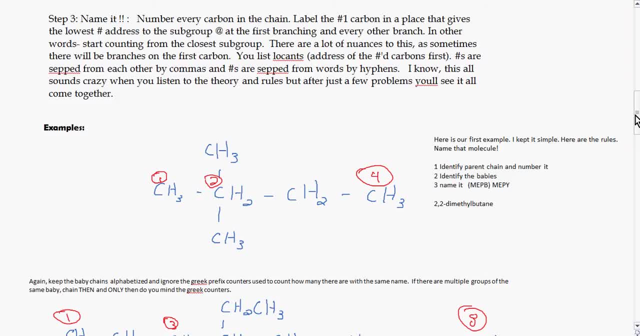 at the first branching and every other branch, So in other words, start counting from the closest subgroup. There are a lot of nuances to this, as sometimes there will be branches on the first carbon. The address of the carbons are called locants. 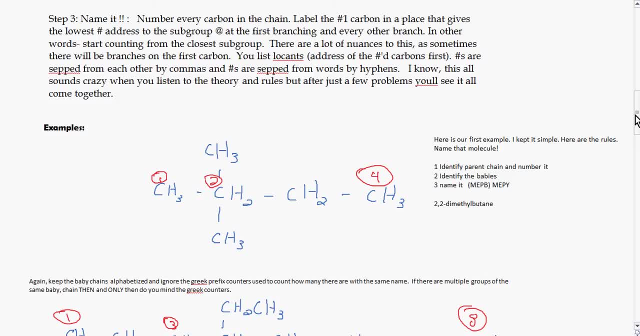 I don't know if that's important or not. Numbers are separated from each other by commas and numbers are separated from words by hyphens. I know, I know this is all sounding crazy when you listen to the theory and the rules. 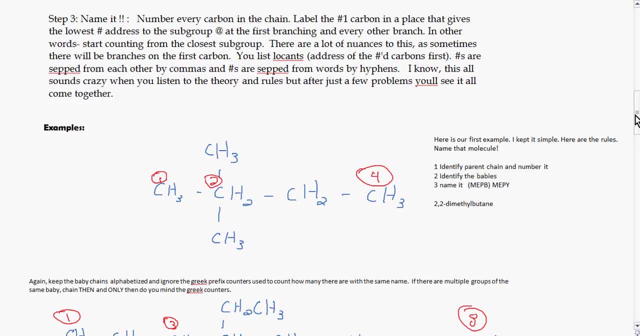 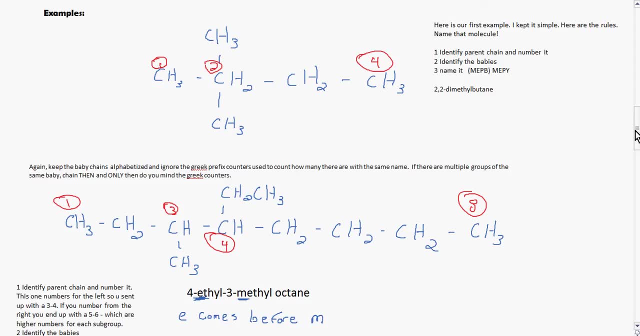 but after a few problems you'll see it all come together. So here is our first example. I kept it simple and I listed the rules. So identify the parent chain and number it, identify the subgroups and then name it. 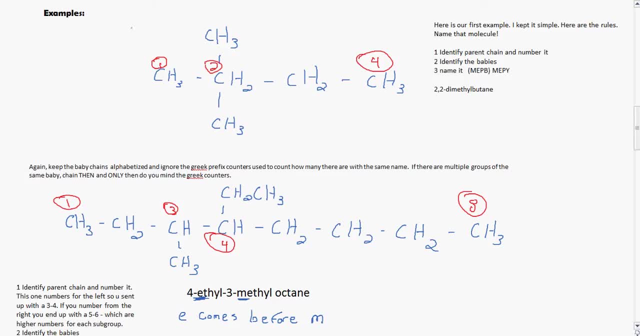 So this first one here is called 2-2-1.. Now you want to start labeling from this carbon right here as your number one, because then your subgroups are on carbon two, which would give you the lowest address for your subgroups. 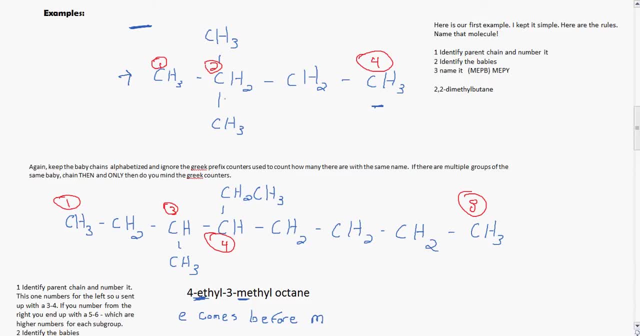 If you start from this carbon here, it would be 1-2-3.. So that gives you the right answer. well, not the right answer, but the right direction. to count from this side so that you have your subgroups at two. 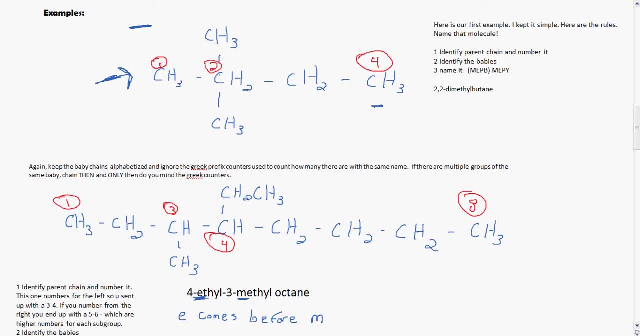 If you have two subgroups on the same one, you just list the number twice with a comma separating the numbers. So this is 2-2-dimethylbutane, because you have your second carbon here and then you have two methyls. 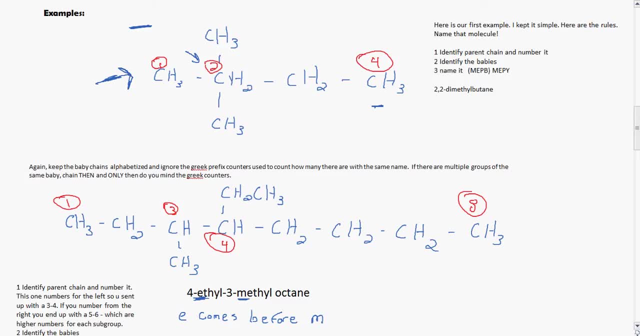 Oftentimes it may help you out to look at the name of the molecule and go backwards. You will get problems where it's just the name and you'll have to draw it. So if you go backwards- let me switch colors here- do this in red. 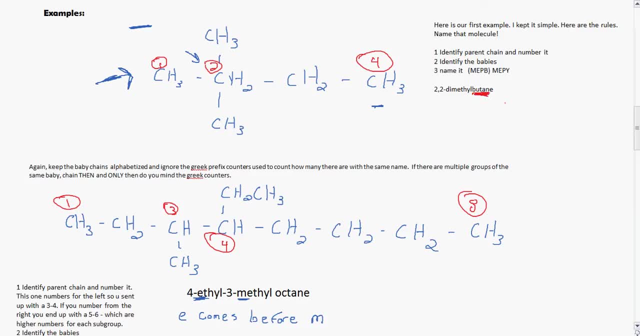 If you go backwards and look at the name, you'll start with butane. so MEPB, you know it's a four-carbon chain. And then, moving one step further, dimethyl. you know that there's two methyl groups And then 2-2, you know both those methyl groups are on the second carbon. 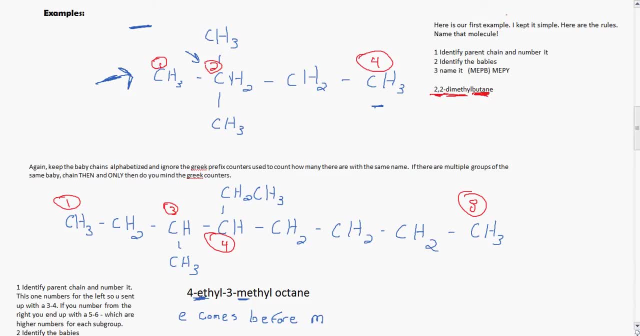 So you can think of it that way as well, looking backwards. So again, keep the baby chains alphabetized and ignore the Greek prefixes used to count how many there are with the same name If there are multiple groups of the same baby chain. 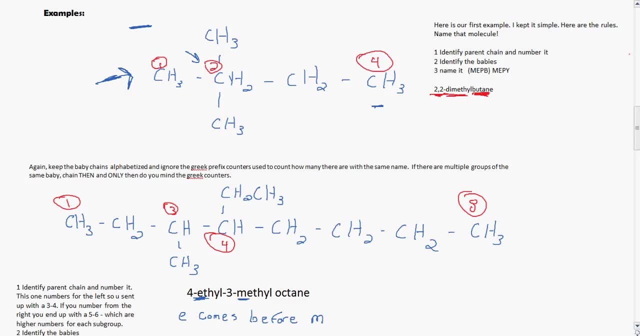 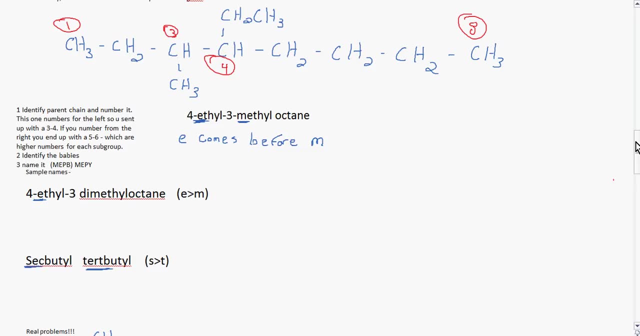 then, only then, do you mind the Greek counters? So let's move on to another example. Here you have 4-methyl-3-ethyl-octane, So again, identify the parent chain and number it Again. on this side you're going to start counting from the 1 on this side. 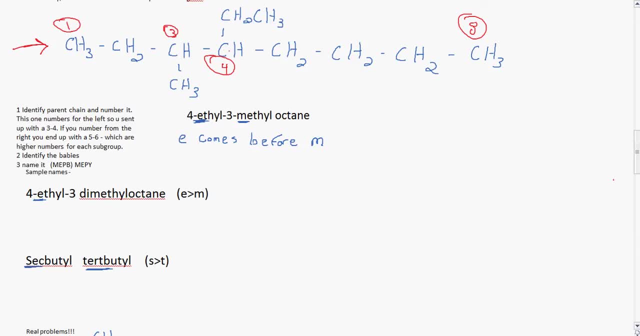 because that gives your first locant as a 3 and your second as a 4.. If you count from this other side, you would have 1,, 2,, 3,, 4, and then this would be 5 and 6 instead of 3 and 4.. 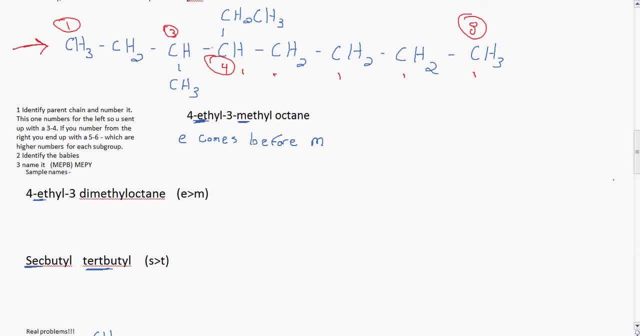 Again, you want to keep those numbers low, for each address, for each position. So you're going to number from the left and you end up with a 3, 4.. So then you identify the chains On carbon 3, you have a methyl group. 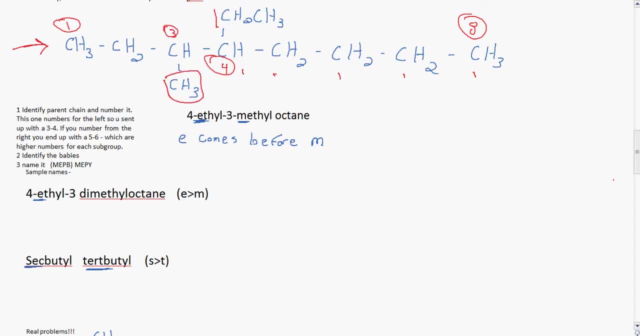 Methyl, because it's one carbon, And on carbon 4, you have an ethyl group- Ethyl because it's two carbons, And again you name them alphabetically. So this is going to be named 4-ethyl-3-methyl-octane. 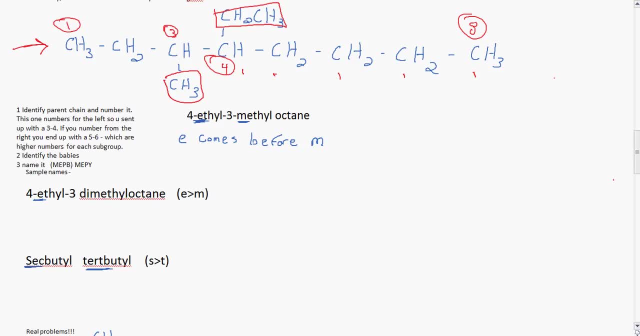 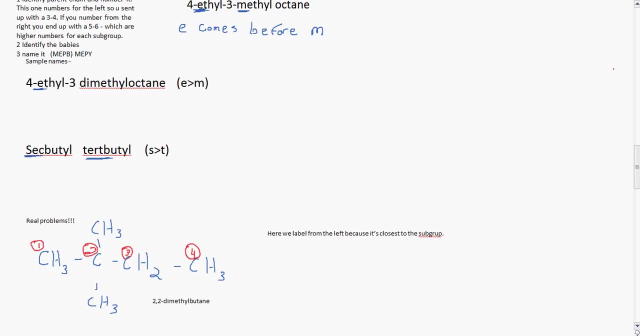 And you can clearly see why it's an octane: because it has 8 carbons and that's your longest chain. Here are some examples. These are just names. I didn't draw these out, But just so you can see how the names go. here you have 4-ethyl-3-dimethyl-octane. 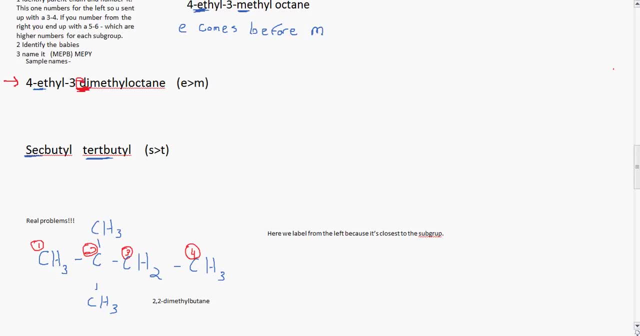 Since it's ethyl-methyl and you don't count these Greek letters, so you can, even though you need to put it in there. E comes before M. You should know the alphabet by now. Secbutyl and tertbutyl. here's one where, when you're counting the exact same group, then 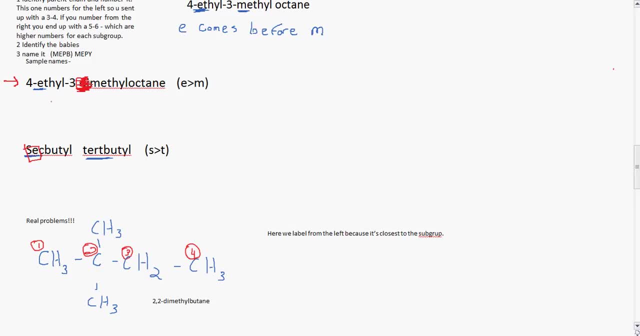 the counters matter. So if you're counting a bunch of methyls or a bunch of ethyls- and they're all ethyls, then these matter. So here is secbutyl would come before tertbutyl, So this was like 2-secbutyl and then maybe- I don't know- this was 4-tertbutyl. 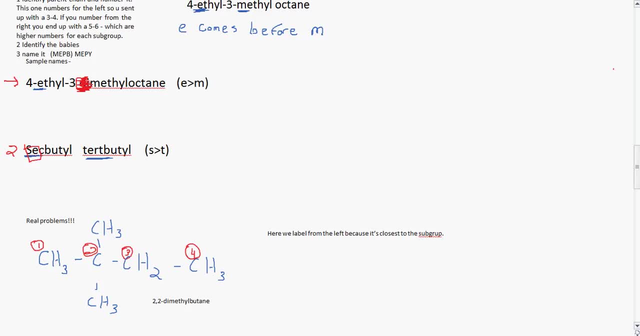 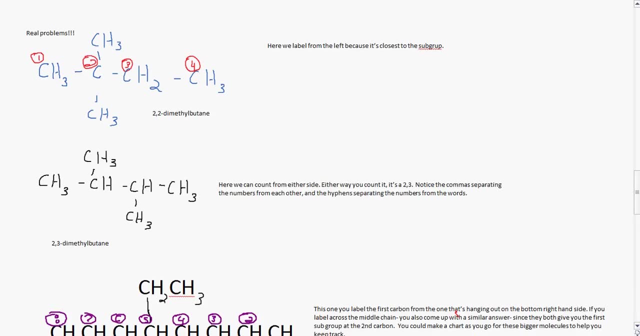 Sec would come before tert because S comes before T. So moving on, here's some real problems. Now in 2-2-dimethylbutane. we already looked at this and we labeled from the left because it's the closest subgroup. 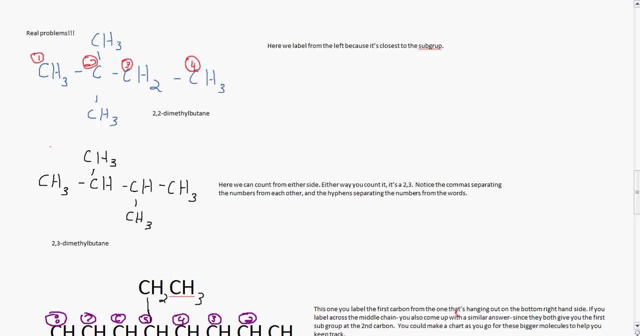 Moving on to 2-3-dimethylbutane. Okay, Dimethylbutane. Lost my cursor here. Oh, here it is This guy right here. Here you can count from either side, and either way you count it, it's going to be a 2-3.. 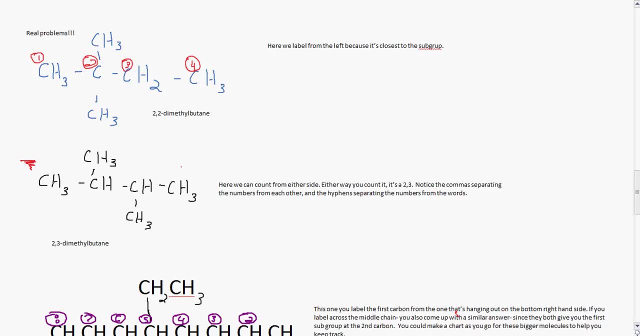 And notice the comma separating the numbers from each other and the hyphen separating the numbers from the word. So it's 2,3-dimethylbutane. Now, this is this sort of has a plane of symmetry. you can, I don't know, maybe not. 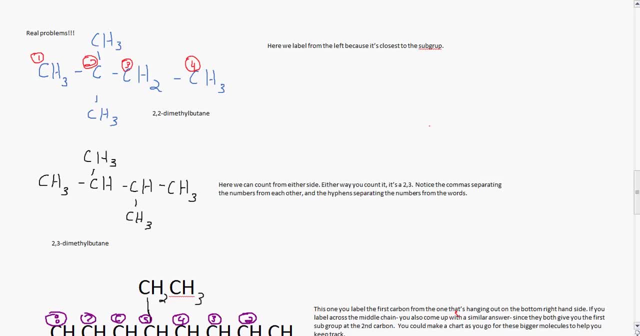 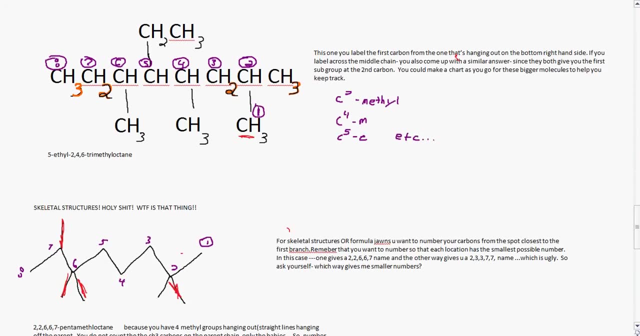 But you can see that it doesn't matter. if you count from either side, you'll have a 2-3.. Okay, So moving on. next, This one you can label from the first carbon, from the one that's hanging on the bottom. 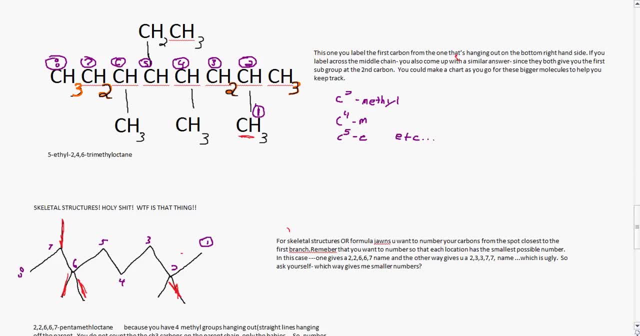 right side. If you label across the middle chain, you'll also come up with a similar answer, since they both give you the first subgroup at the second carbon, And you can make a chart as you go for these bigger molecules to help you keep track. 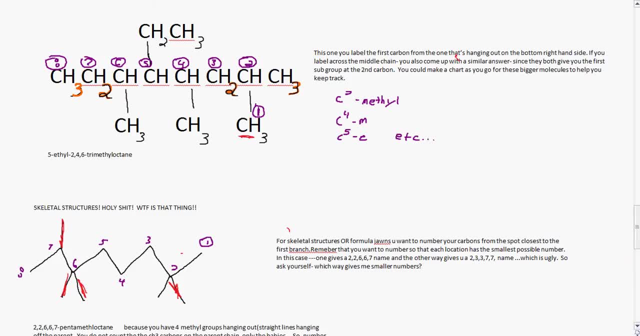 So if you label from here as your 1,, you'll have 1,, 2,, 3,, 4,, 5,, 6,, 7, 8.. So on your 2 right here, And on carbon 2, if this was a bond, you would have C2-methyl. 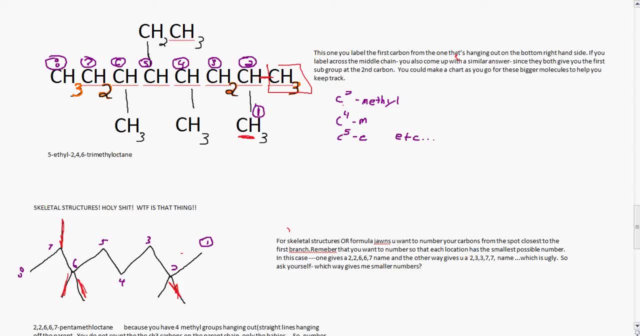 On C4 you have a methyl, On C5 you have an ethyl, etc. So you can make a little chart here like that, like I do, just to keep track, and then name it. So this would be 5-ethyl and then 2,, 4,, 6-trimethyl-octane. 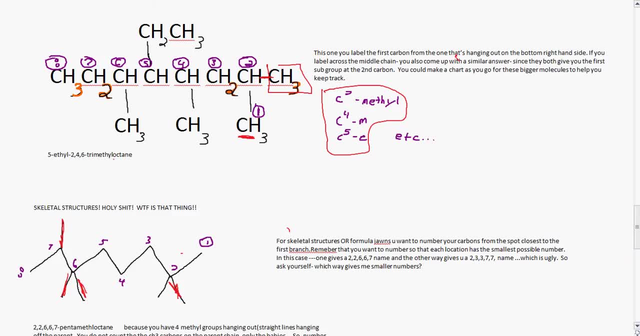 Because on 2,, 4, and 6 you have methyl groups. So again reading that backwards Octane, you have 8 carbons Trimethyl, you have 3 methyls And then you have 2,, 4,, 6-octane. 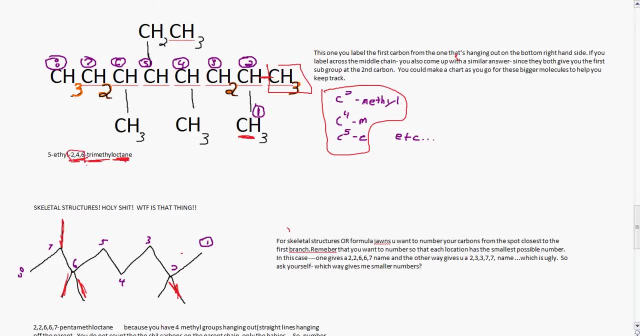 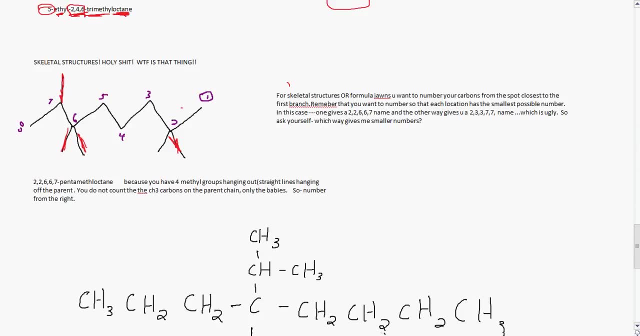 And then you have methyl groups that are attached to number 2,, 4, and 6 carbons. Then you have an ethyl group attached to the 5th carbon. So let's look at a skeletal structure, because you'll see a lot of these that you have to. 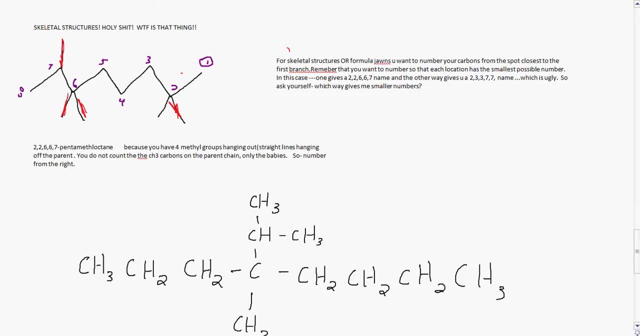 name as well, And for skeletal structures or formulas. again, you want to number your carbons from the spot closest to the first branch. So remember that you want to number each location and have the smallest possible number. In this case, if you number with the 1 on the right, 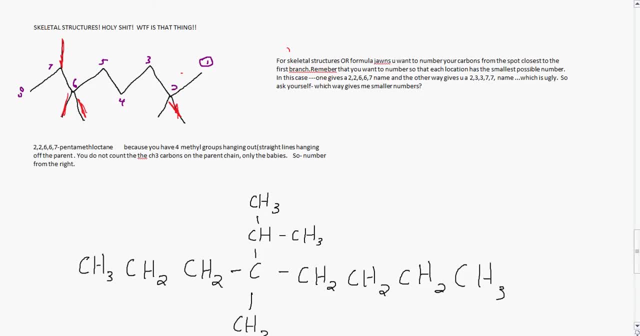 It will give you a 22667.. And the other way gives you a 23377 name, which is ugly. So ask yourself which way gives me the smallest numbers. So you want the 22667, because the second position here is a 2.. 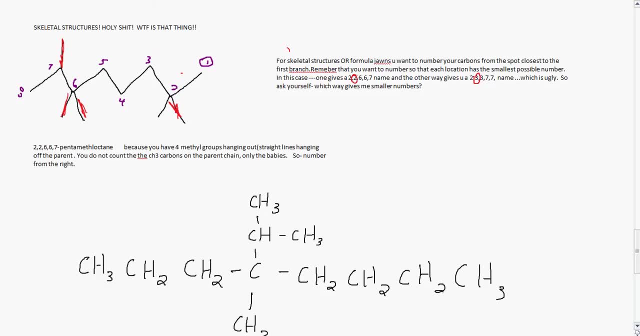 And the second position here is a 3.. So you want to go with the 2, because that's a smaller number for the second position. So naming: here: you see you have a 1, 2. And then hanging off is 2 or 2 methyl groups. 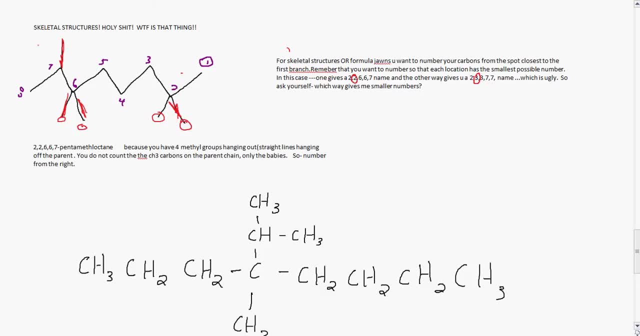 3,, 4,, 5, 6.. Hanging off is 6 or 2 methyl groups, And then the 7 is 2.. And then the 7 is 2. And then the 7 is 2.. And then there's another methyl group. 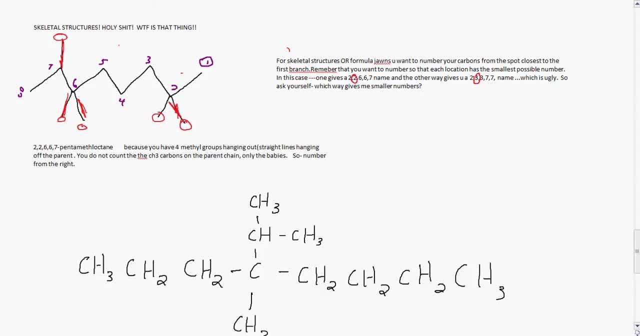 So 22667 tri, No 22667, pentamethyl octane, since there's 5 methyl groups, Because you have the 4 methyl groups hanging out off the parent chain And you don't count the CH3 carbons on the end of the parent chain. if you see it in a formula, 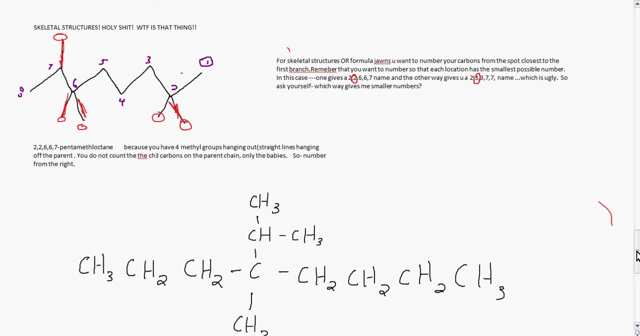 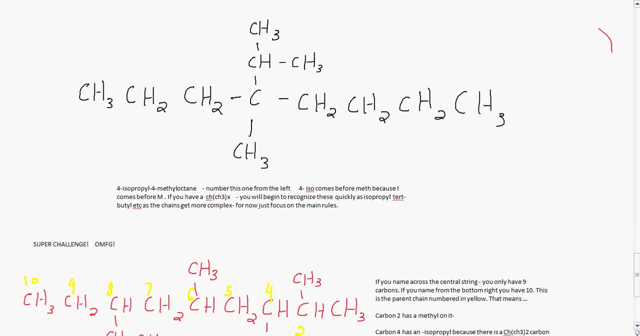 So number from the right And looking at, I think it's our last one, Nope 2 more. This one is 4 isopropyl 4 methyl octane And this one you're going to number from the left, from this side, for obvious reasons. 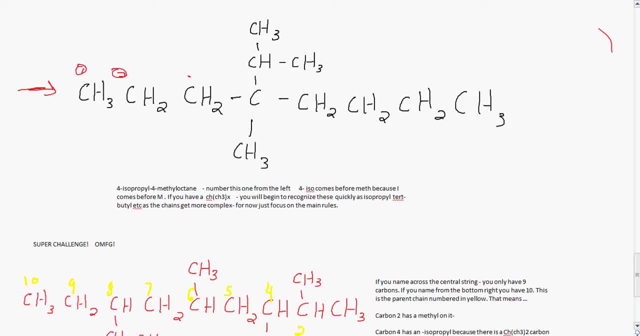 If you count from this side, you have 1,, 2, this one's 3, and this one's 4.. If you count from the right side, you'll have 1,, 2,, 3, 4, then that one's 5.. 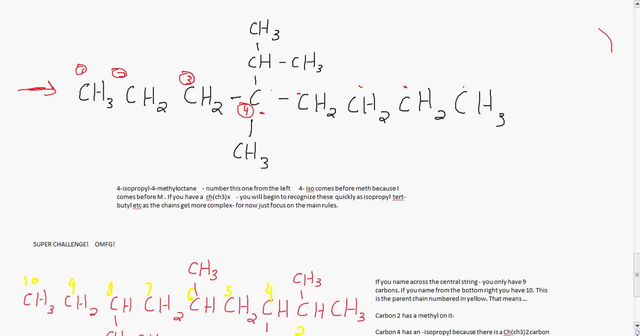 So that would give you the lowest number for the location of the first group. So you're going to number from the left And 6,, 7,, 8,, 9.. Well, 8.. So you have 8 carbons here. 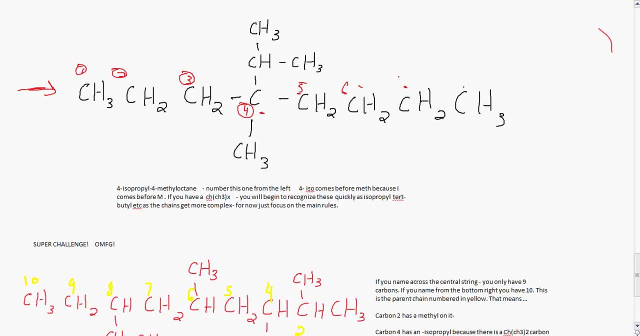 4,, 5,, 6,, 7, 8 carbons And 4 iso comes before meth, because I comes before M, And if you have CH, CH3X- it's this little formula down here- You're going to see a CH with CH3s attached. 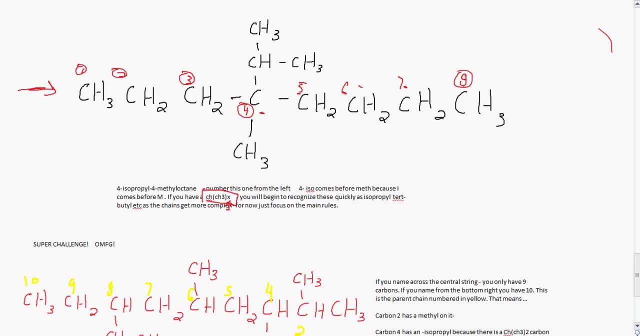 And then the number of the CH3 is going to vary, that methyl group. You'll begin to recognize these quarks. You'll start to recognize them very quickly as isopropyl or secbutyl, etc. as the chains get more complex. 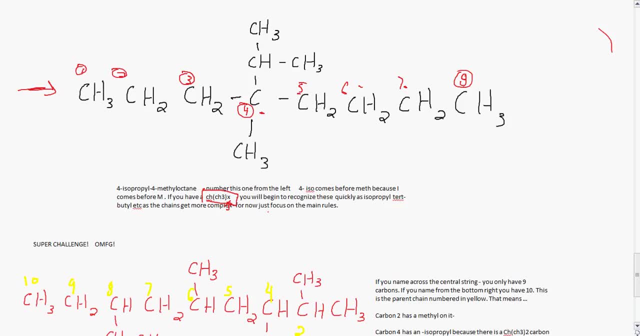 But for now just focus on the main rules of numbering. That's not as important as you get further along. So here is your isopropyl MEP3 carbons, And then here is your methyl So 4, isopropyl 4 methyl octane. 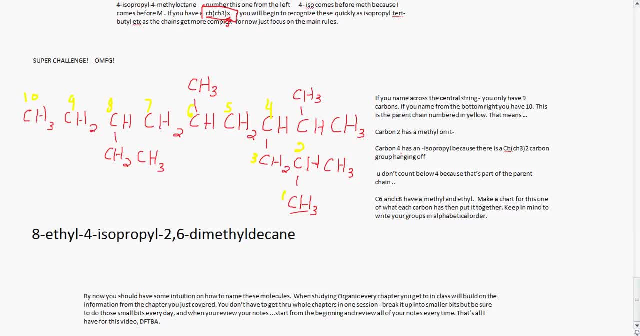 And then coming down here is a much more complex one. So if you name across a central string, you have 9 carbons. If you name from the bottom right, you're going to have 10 carbons, And I numbered them in yellow.